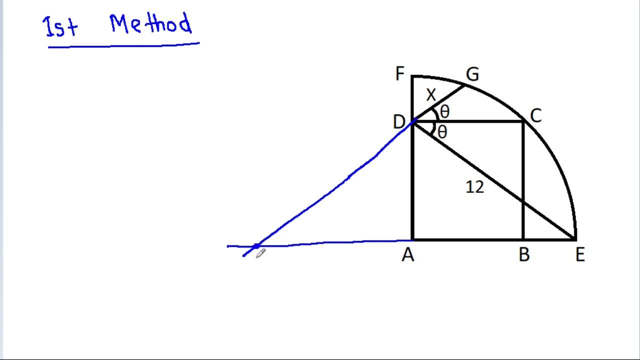 suppose this point is- edge and opposite angles are equal, so this angle will be theta, so these two angles will be also equal. they will be 90 degree minus theta, 90 degree minus theta, and these angles will be 90 degree. so in triangle DHA and triangle DEA. 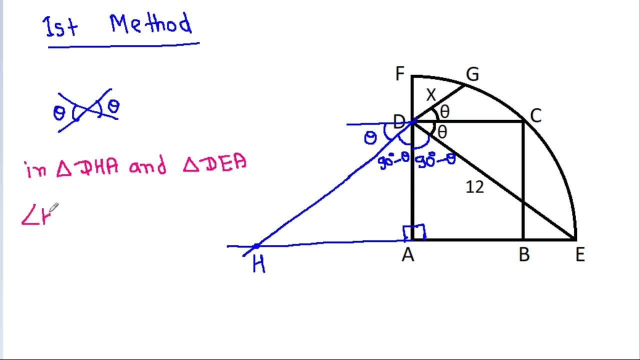 angle HAD is equal to angle EAD. DA is common and angle HDA is equal to angle EDA. So triangle DHA- it will be congruent to triangle DEA. DH it will be equal to DE and DE is 12, so DH will be 12,. 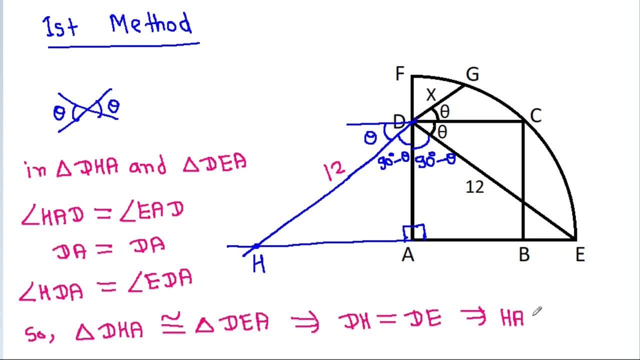 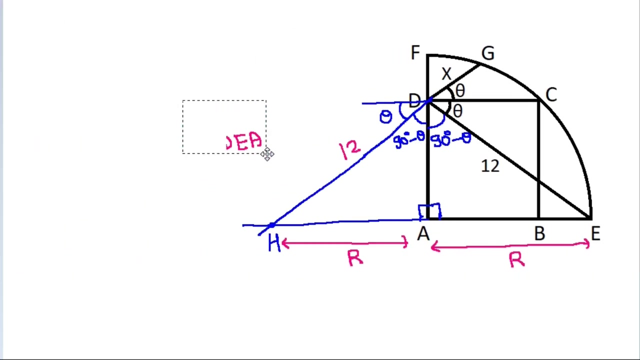 and also HA, it will be equal to EA, and EA is radius of quarter circle, so h, a will be radius, and if we join a g, then a g is also radius of quarter circle. and now in triangle, h g, e, h, g, e. this: 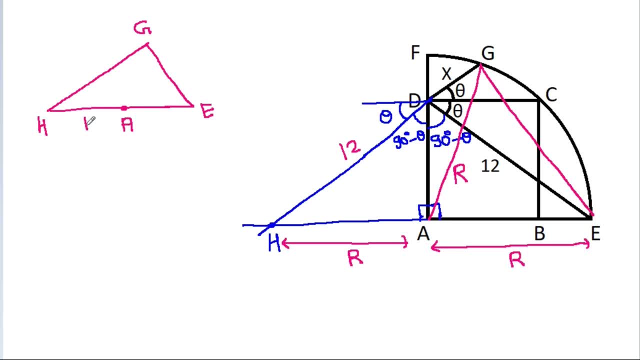 point is a and h. a is radius, a, e is radius and a, g is radius. so point a: it will be circum center of triangle g, h, e. that means we can make a circle around triangle h, g, e and in any circle if a, b is diameter. 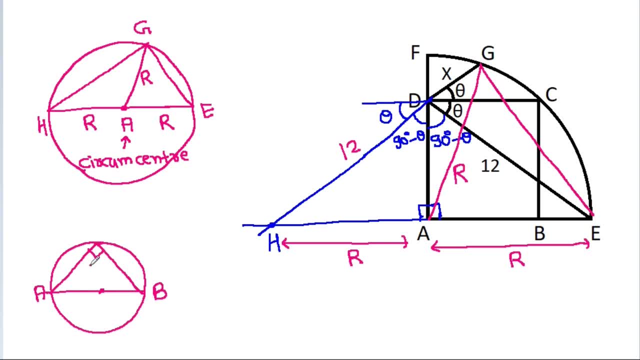 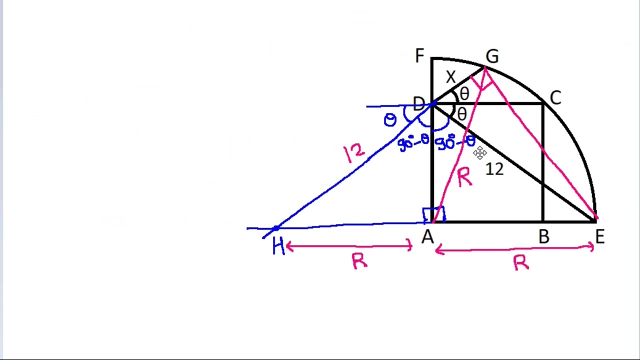 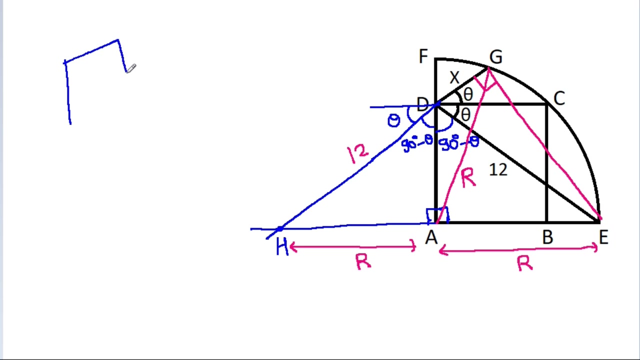 then this angle on the circle, it will be 90 degree. so here this angle will be 90 degree, this angle will be 90 degree and if in any coordinate run a, b, c, d, if this angle is alpha, angle is beta, and if unfa-plus beta is 180 degree, then ABCD, it will be cyclic. 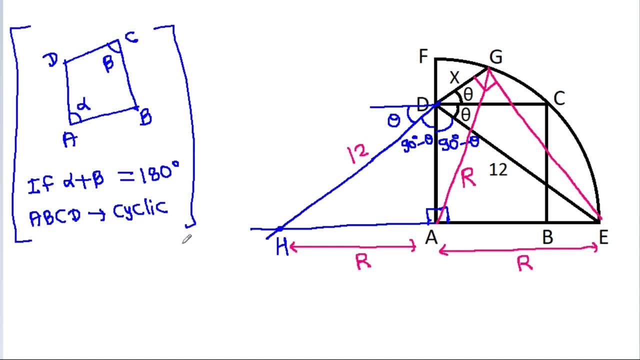 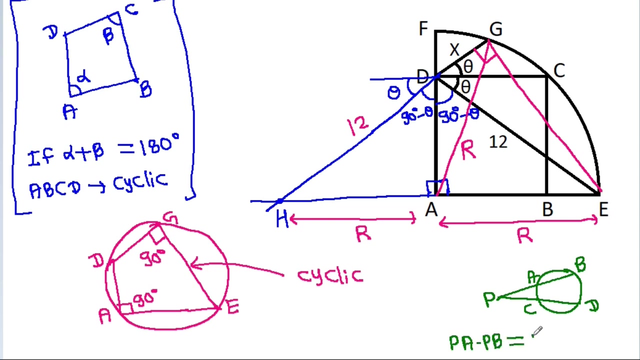 and here in ADGE it is A, D, G, E. this angle is 90 degree and this angle is 90 degree, so ADGE it will be cyclic. that means we can draw a circle around ADGE and in any circle. if this point is P and it is A, B, C, D, then PA times PB it is equal to PC times. 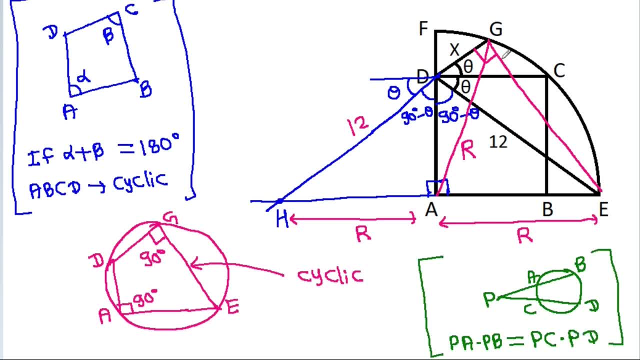 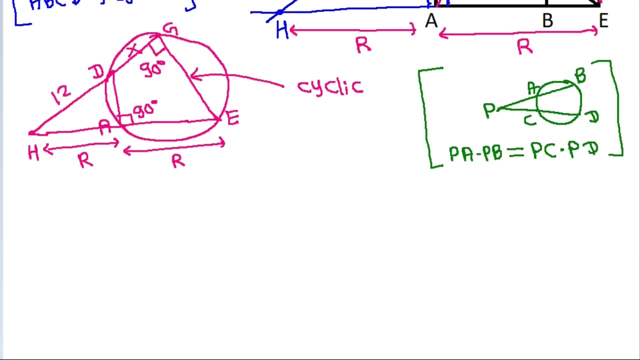 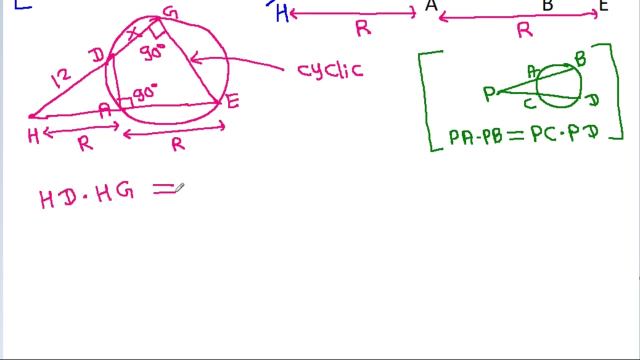 PD, and here this point is H, P and HA is R, AE is R and HD is 12, and DG is X. So HD times HG, it will be equal to HA times HE, And HD is 12 times HG, it will be 12 minus X. it is equal to HA. is R times HE, it will be R minus R. 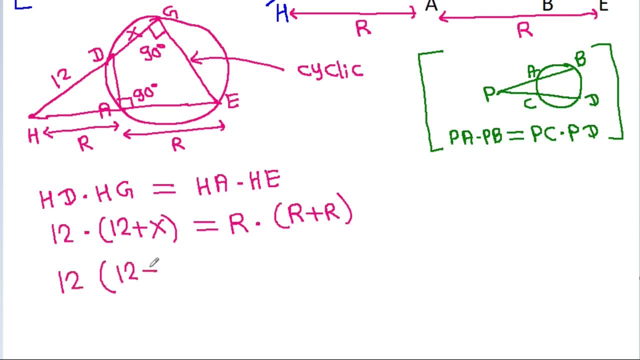 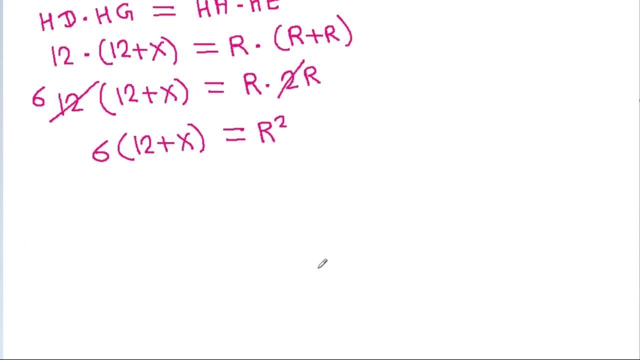 And 12 times 12 minus X is equal to HE. So 12 times 12 minus X is equal to R times 2R, and 2 times 6 is 12, so 6 times 12 minus X it is equal to R squared, and 12 minus X it is equal to R squared by 6.. 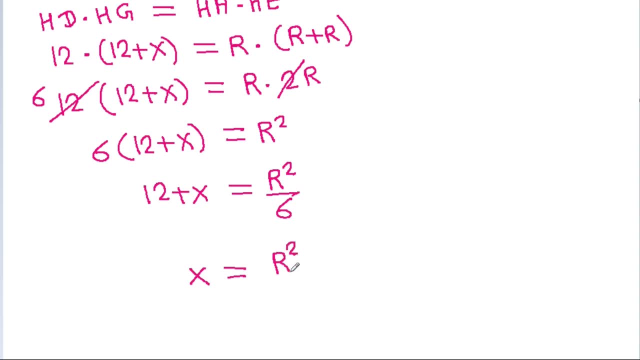 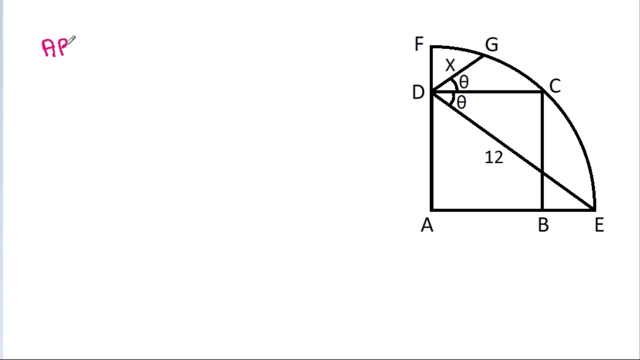 So X will be equal to R squared by 6 minus 12.. And Now ABCD. it is a square, So AB will be equal to BC, will be equal to CD, will be equal to DA. Suppose Y. 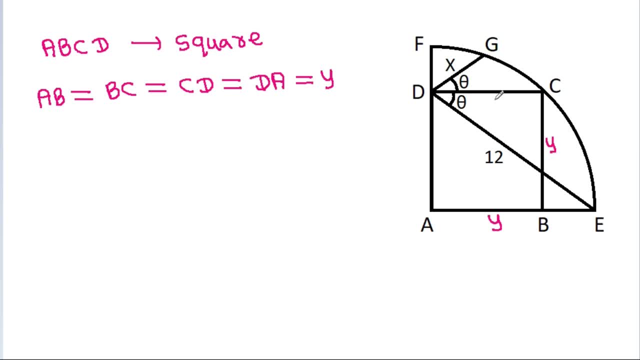 So AB is Y, BC is Y, CD is Y and DA is Y And AE is radius, And these angles are 90 degree. So inter-angle D is 90 degree. So inter-angle D is 90 degree. 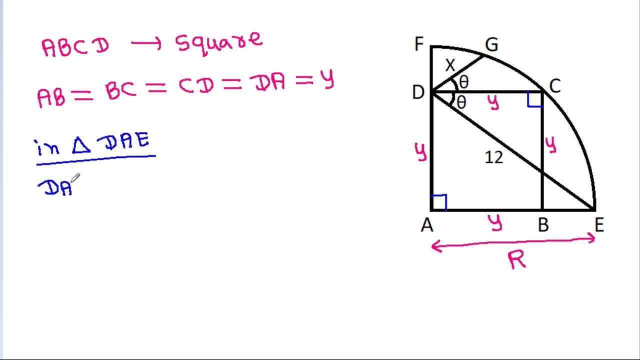 Suppose DAE, DA square minus AE square, It will be equal to DE squared. And DA is Y squared minus AE is R squared, it is equal to DE is 12 squared. and if we join AC, then AC will be radius and also AB square minus BC square it will be. 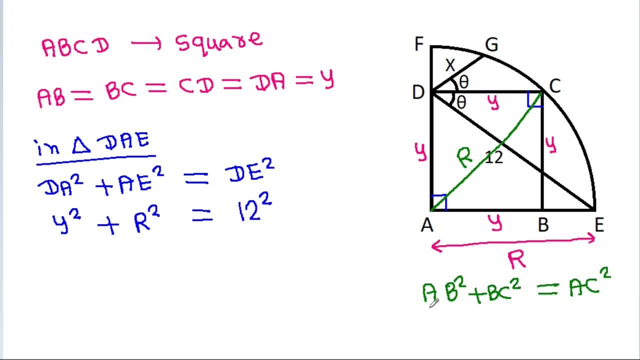 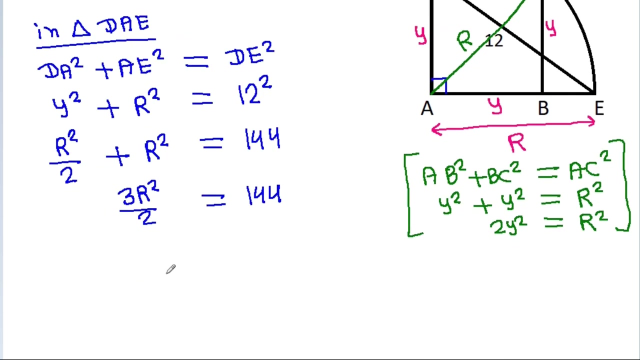 equal to AC square and AB is y square minus BC is y square. it is equal to AC is radius square. so 2y square will be equal to r square. so y square will be r square minus r square will equal to 144.. and it is 3r square by 2 is equal to 144. 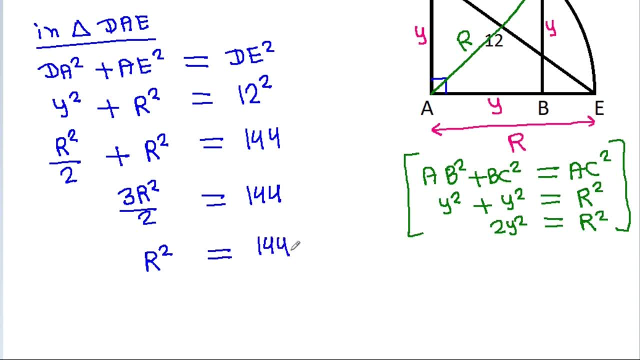 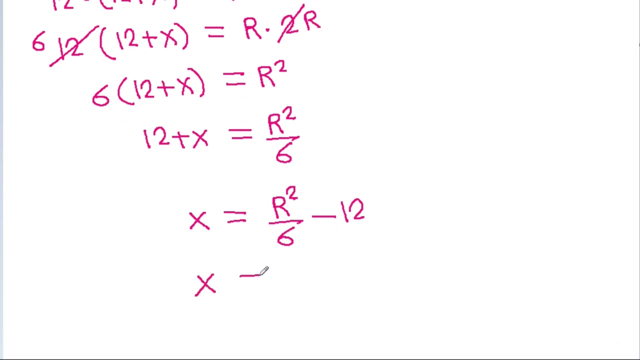 r square will equal to 144 times 2 by 3 is equal to 144, and 3 times 48 equals to 144, and 1 is equal to 144. so 3 times 48 equals to 144. 48 times 2 is 96. So x will be equal to R. square is 96 by 6 minus 12 and it is 16. 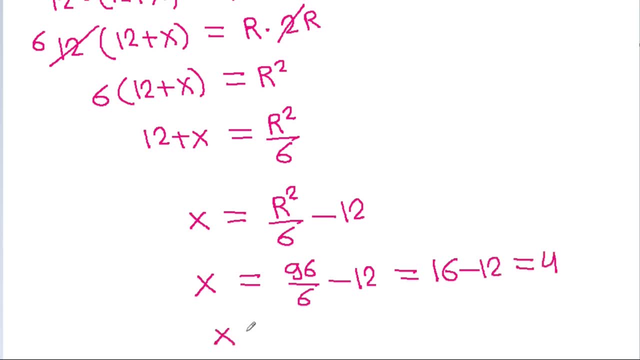 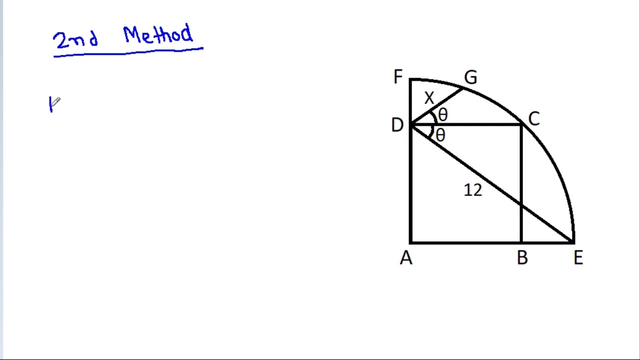 minus 12. That is 4.. So x is equal to 4.. And second method, We have AE. It will be parallel to R square. We have DC, So this angle will be also theta And this angle is 90 degree. And if we draw a perpendicular from G on AE, 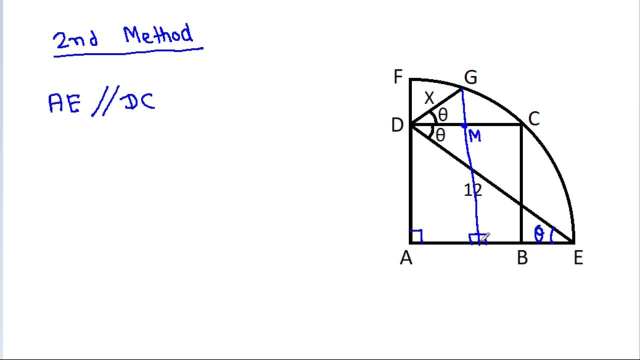 Suppose this point is M and this point is DC And this point is N, Then here this angle is 90 degree. So DM, It will be equal to x cos theta, And it is equal to x And inter angle DAE cos theta. 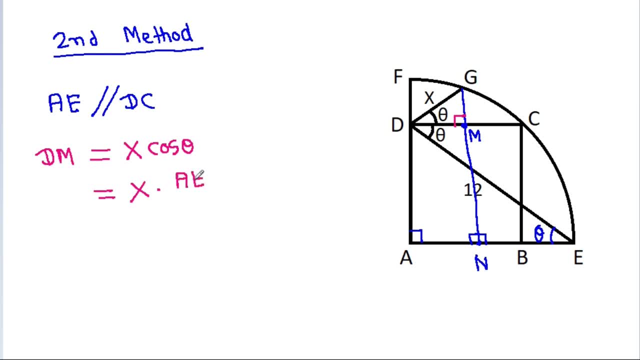 It will be equal to x cos theta, So it will be AE by DE. And AE is radius, So it will be equal to x times R, by DE is 12.. And AN it will be equal to DM, That is, x times R by 12.. 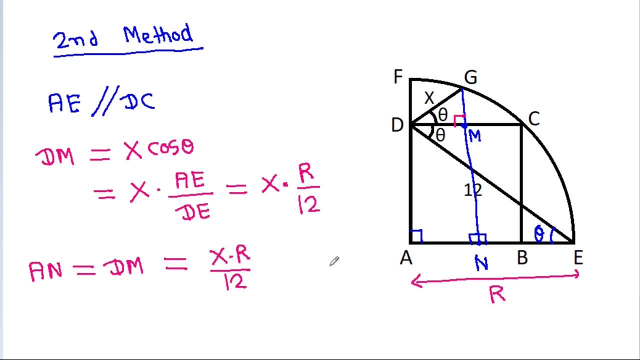 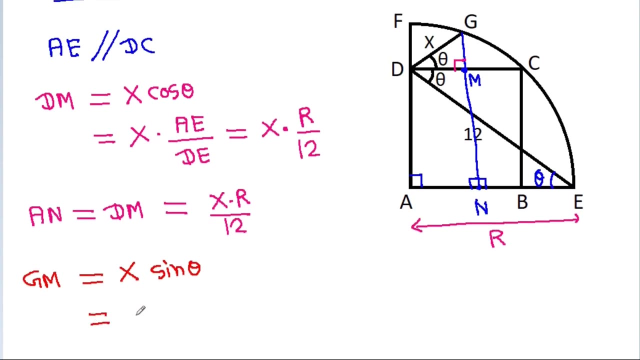 And also GM. It will be equal to x sin theta And it is equal to x times And from here sin theta It will be AD by DE And AD is y. So it will be x times y by 12.. So AN, it is xR by 12.. 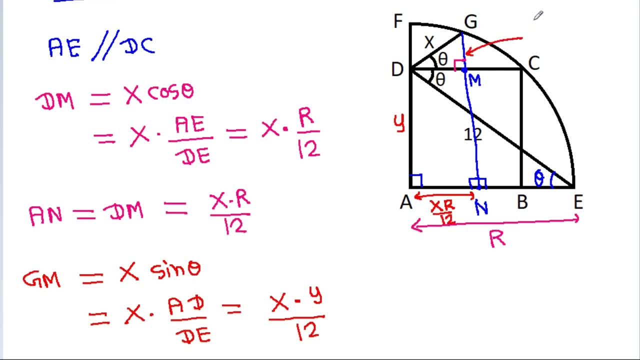 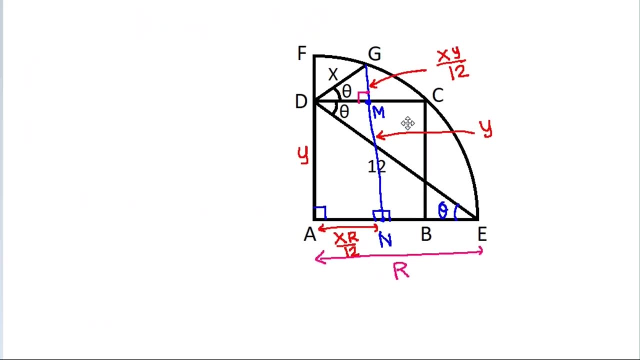 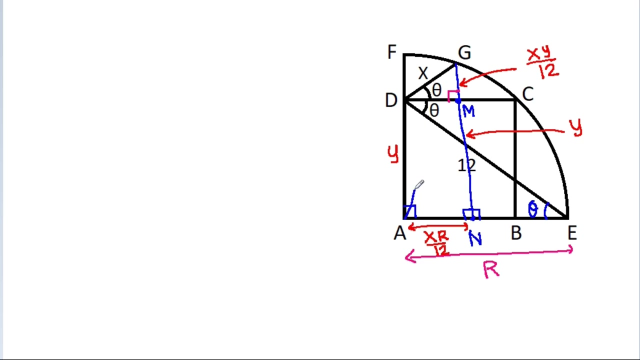 And GM is xY by 12.. And MN It is xR by 12.. And MN is y. So to security. Now you can also see We have the love triangle Again. if you incorporate them this term, Everyone knows the value of the w or the y. 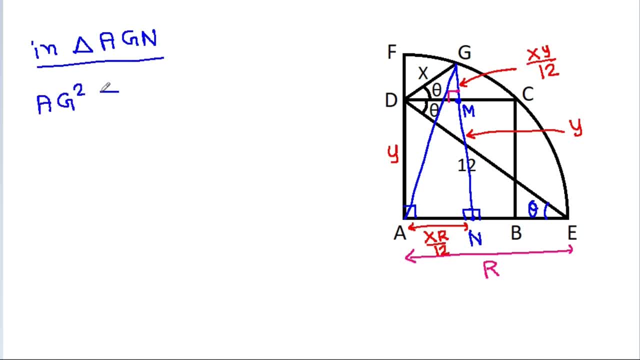 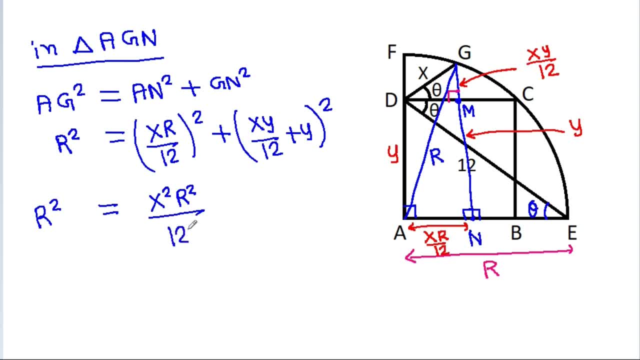 x square, r square by 12 square minus, and It is y square times x by 12 plus 1 square, and a c is radius and a c square is equal to a b square minus b c square, so r a square will be equal to y square. 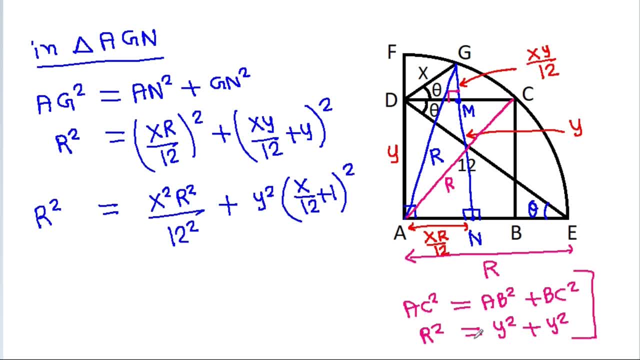 to y square minus y square, So r square is 2y square. It is equal to x square times 2y square by 12 square minus y square times x by 12 minus 1 square, And y square will get cancelled. 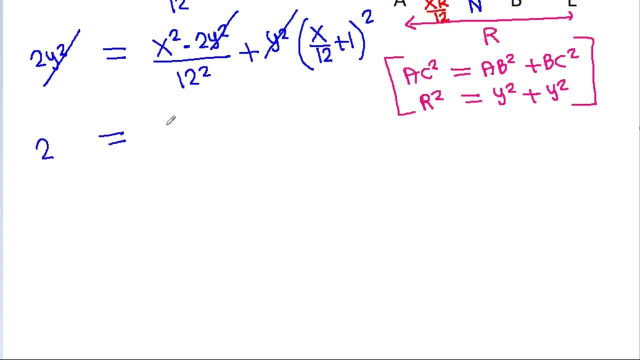 So 2 is equal to 2x square by 12 square minus, and it is x minus 12.. So 2 is equal to 2x square by 12 square, And 2 is equal to 2x square by 144 minus x minus 12. 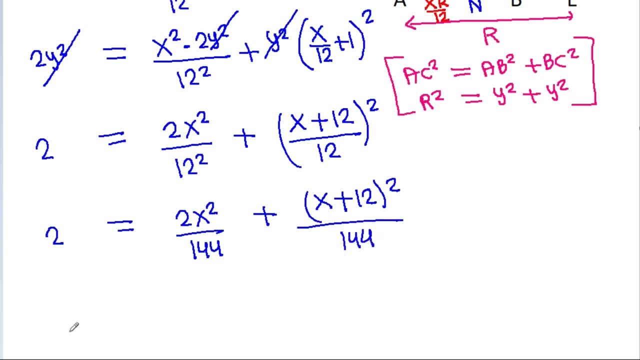 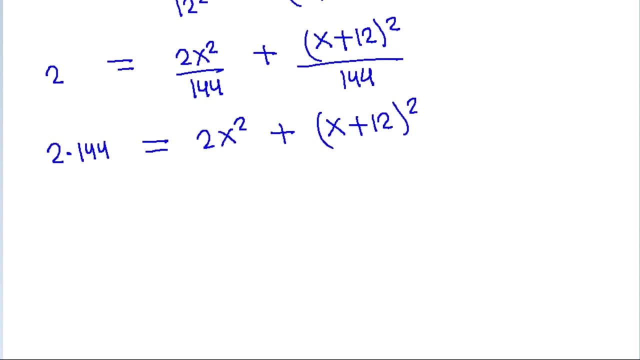 square by 144.. And 2 times 144, it will be equal to 2x square minus. x minus 12 square, And it is 288, is equal to 2x square minus, and this will be x square minus 12 square. 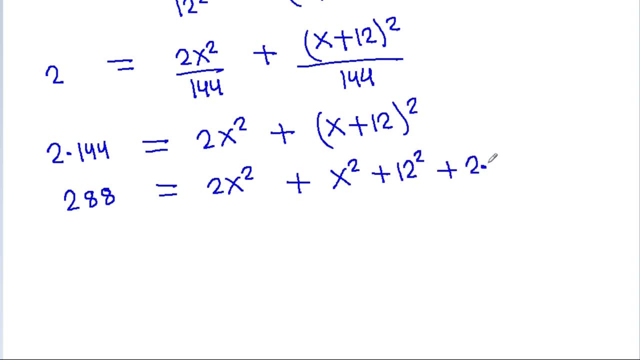 minus 2 times x times 12.. And 288 is equal to 2x square minus x minus 12.. And 288 is equal to 2x square minus x. square is 3x square plus 144 plus 24x, And 3x square plus 24x and 144 minus 288. 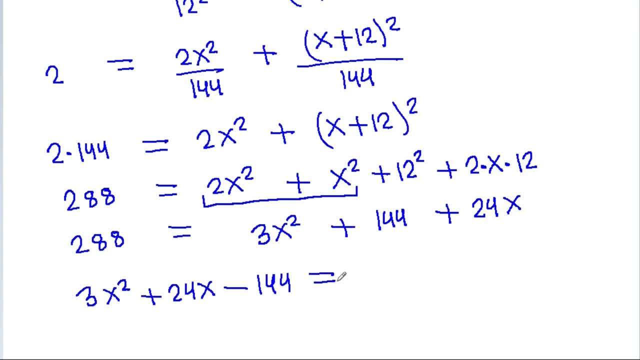 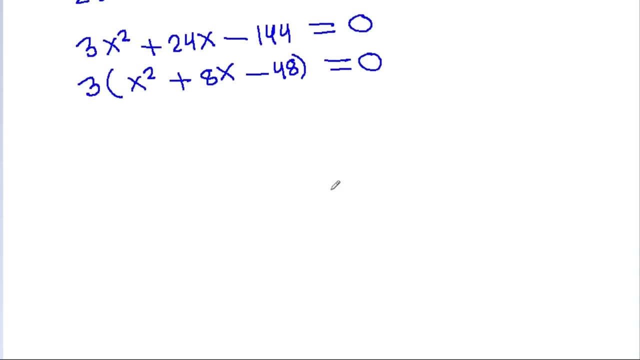 will be minus 144.. It will be equal to 0.. And it is 2x square minus x minus 12.. And it is 3 times x square minus 8x minus 48 is equal to 0.. So x square minus 8x minus 48, it is equal to 0.. And x square and 8x, it is plus 12x. 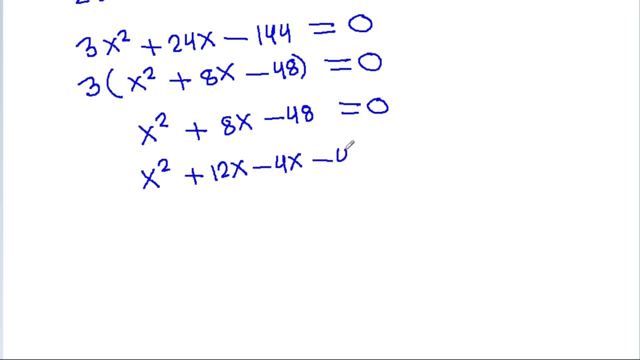 minus 4x minus 48 is equal to 0. And it is x times x plus 2n minus 4 times x plus 2n is equal to 0. And x minus 4 times x plus 2n is equal to 0. So either x minus 4 will be: 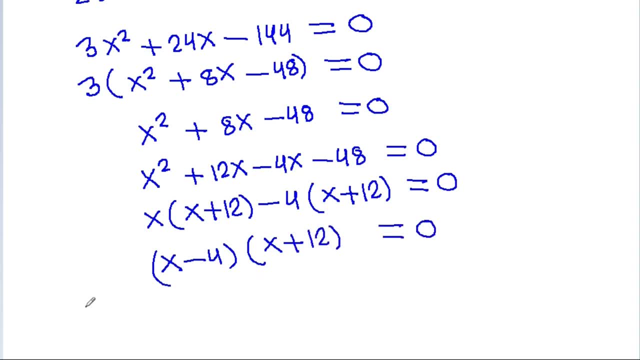 equal to x plus 4, or x minus 4 is equal to 4.. So x is equal to x minus 12x minus 4x is equal to 0. that means x will be equal to 4, or x plus 12 will be equal to 0, so x will be equal to minus 12. 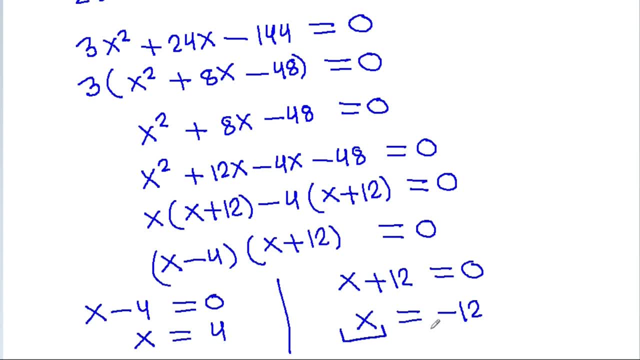 but x cannot be negative, so x cannot be equal to minus 12, so x is equal to 4. you. 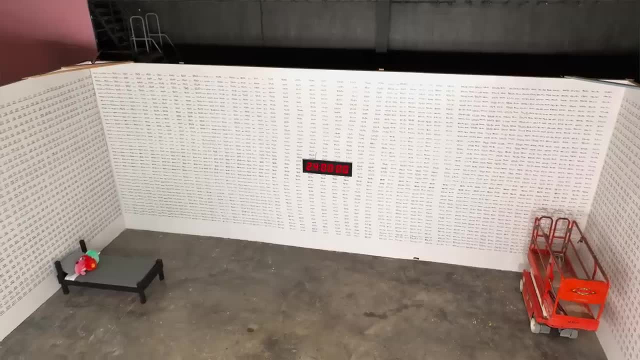 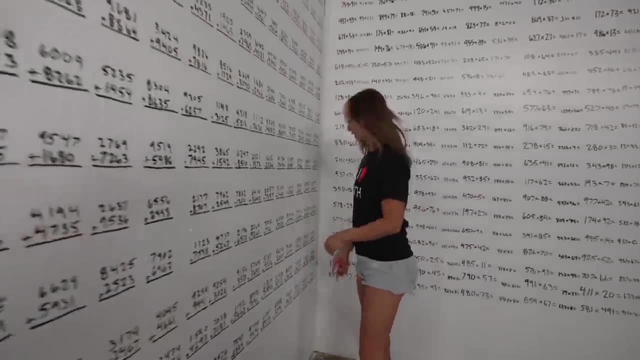 I have 10,000 math problems and only 24 hours to solve them. There are flashcards, workbooks, whiteboards and walls full of math problems, And I'm going to solve every single one of them, starting with this one. 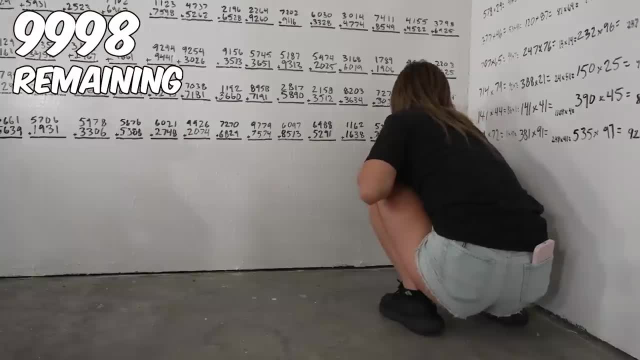 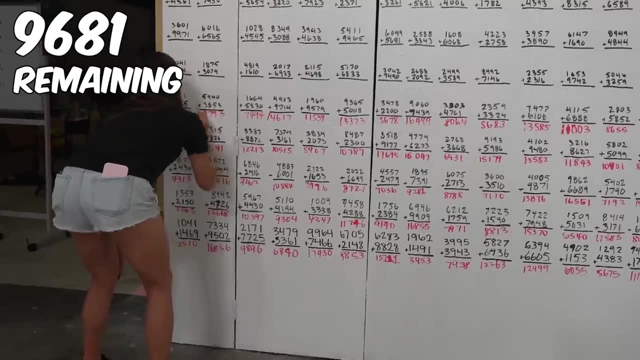 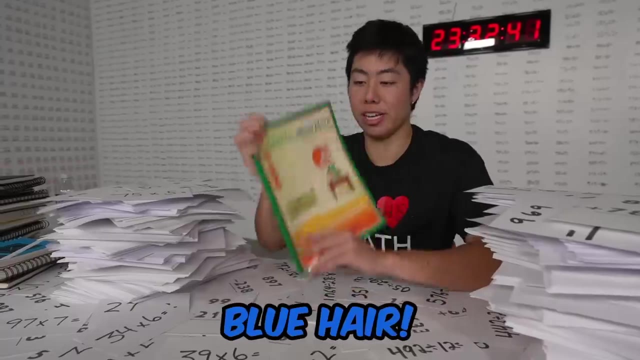 Wow, these are actually really hard. Two, three Editors. can we get a time lapse? 319, 320.. Hey Zach, if I don't complete every single problem in 24 hours, I will dye my hair blue. Blue hair- blue hair, blue hair. 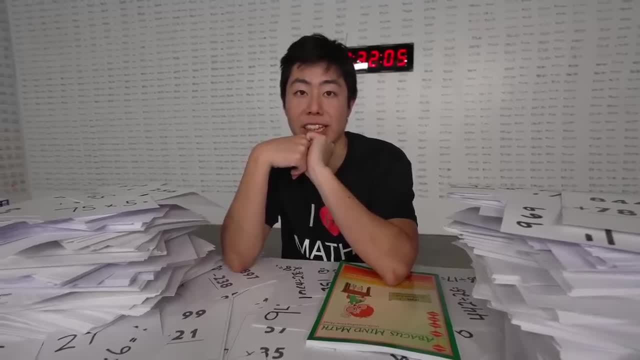 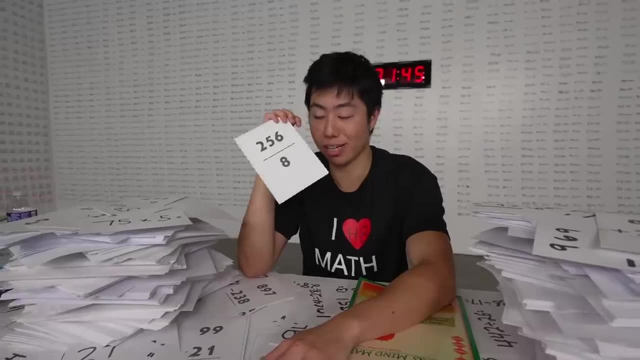 324.. Not really sure how Michelle's gonna complete 10,000.. Last time when she did a 10,000 digit math problem, it was 10,000 numbers. This is 10,000 problems, So she's gonna be writing a lot more than 10,000 digits. 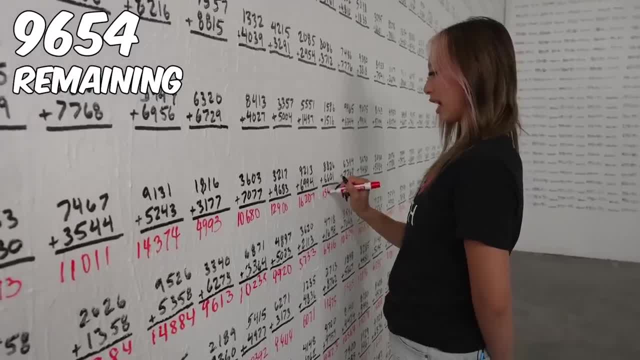 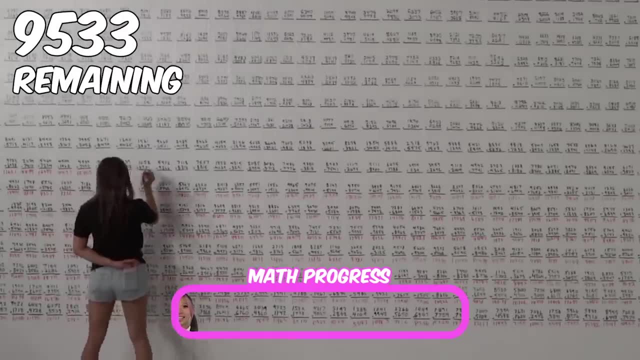 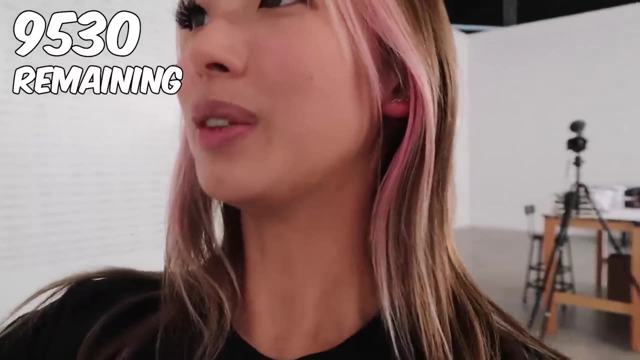 This is actually quite relaxing. I'm confident that I will finish. My head hurts looking at this. 468, 469.. This is what I see right now. Blurry, There's just so many math problems, All right. 471, 472.. 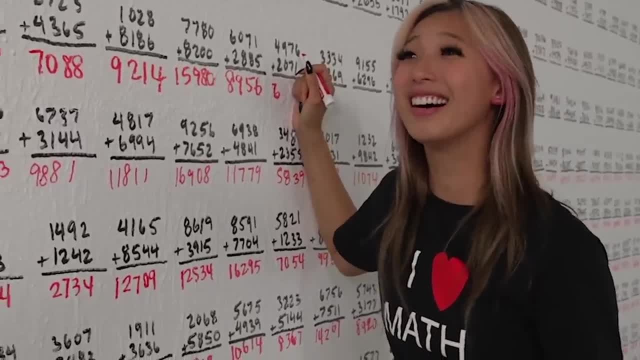 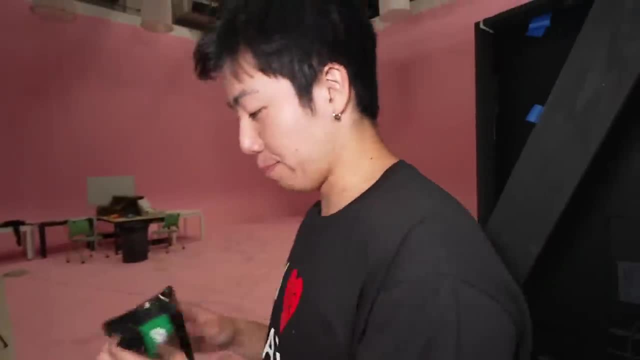 Oh no, Zach, I got something wrong. Does something happen? Every time I get something wrong, I have to do a punishment. I will be right back. Wait what? Here's the completely random punishment. I did not just choose this off the table.